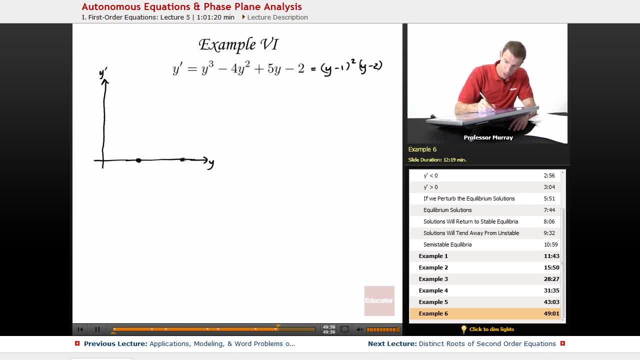 We had roots at y equals 1 and y equals 2.. And then we had a curve that just goes up and just barely touches at y equals 1, and then it goes back down again and then it goes up through y equals 2.. 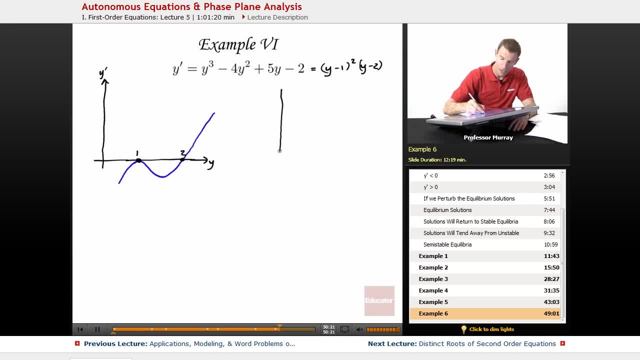 And we've got to translate that into a graph of solutions in terms of y and t. So remember, when you're doing a graph of solutions, you're going to have to have a graph of solutions. So remember, when you're doing a graph of solutions, you're going to have to have a graph of solutions. 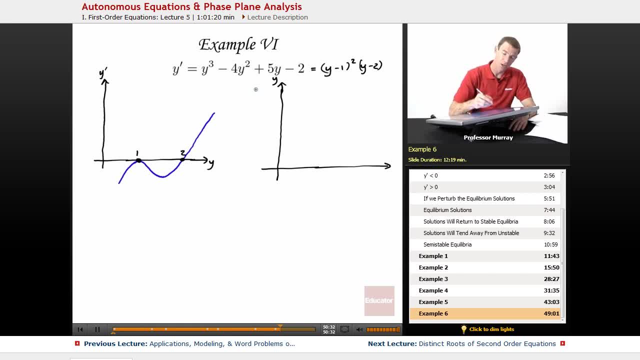 When you're graphing the solutions, y is the vertical axis. When you're graphing the phase plane analysis, y is the horizontal axis. That's always a little confusing, but you want to be very clear to keep track of which graph is which and don't mix them up. 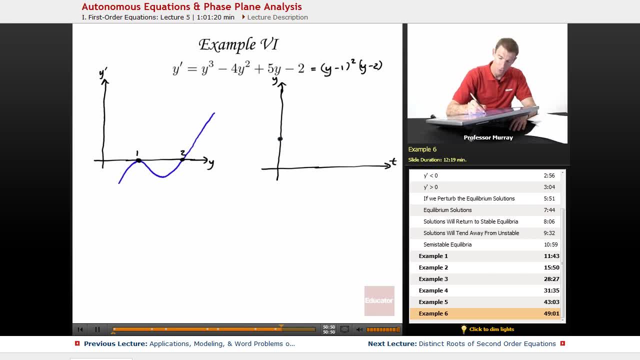 Here I'm going to start by graphing y equals 1 and y equals 2, and those correspond to equilibrium solutions equal to zero. So I'll graph a couple of horizontal lines there. Those were my two equilibrium solutions, And then I want to figure out what the other solutions do. So I'll go back and 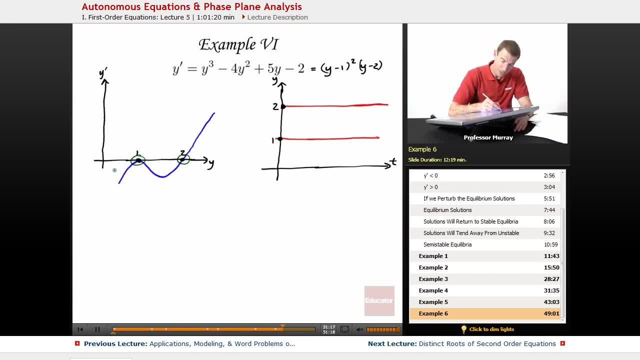 look at the phase plane analysis. If I look down here, when y is less than one, I see that y prime is less than zero because the curve is down here below the axis. When y is between one and two, I still see that y prime is less than zero. And then when y is bigger than, 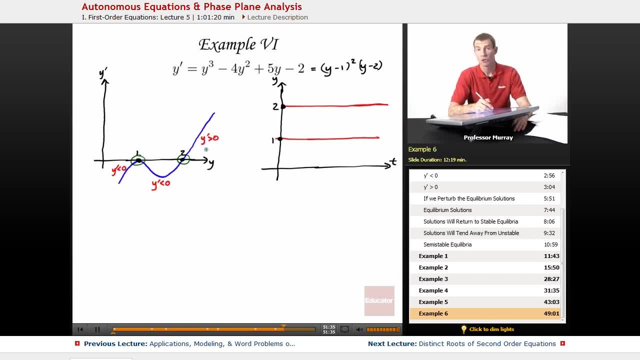 two, I see that y prime is greater than zero, So I'm going to use that to draw my solution curves. When y is less than one, I have solution curves that slope downwards, So I'll draw these curves sloping downwards. When y is between one and two, I still have y prime. 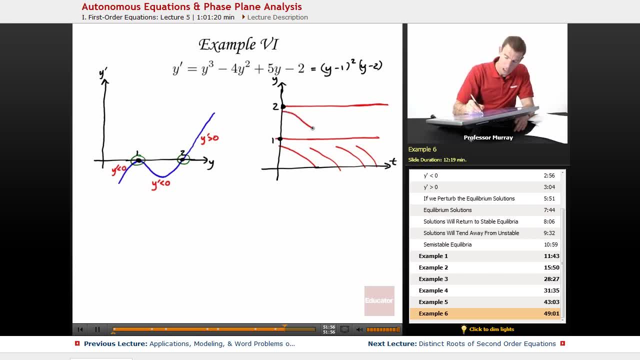 less than zero. so I'm going to draw my curves, still All sloping downwards, leveling off when they get to the equilibrium solutions And when y is bigger than two up in this region that corresponds to this region here. I see that 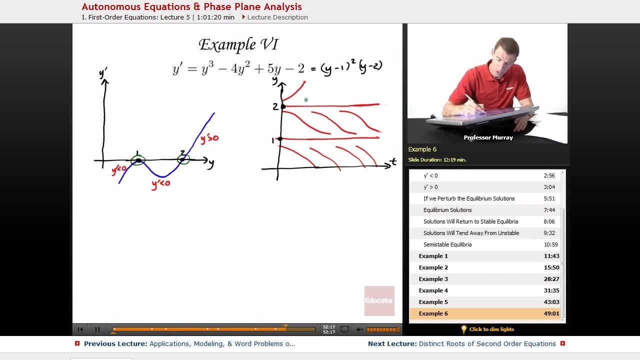 y prime is positive, So I'm going to draw my solution curves positive. So on the strength of that, having drawn these other solution curves, I can label which of my equilibrium solutions are stable or unstable or semi-stable. So if I look at y prime to start with- or sorry, y equals one to start with, that's. 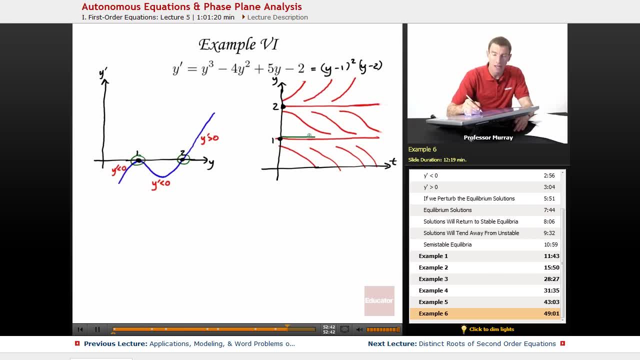 this solution curve. here I see that if it got bumped a little bit, if it got bumped a little bit down, then the solution curves would go far away. If it got bumped a little bit up, then the solution curves would come back and approach. 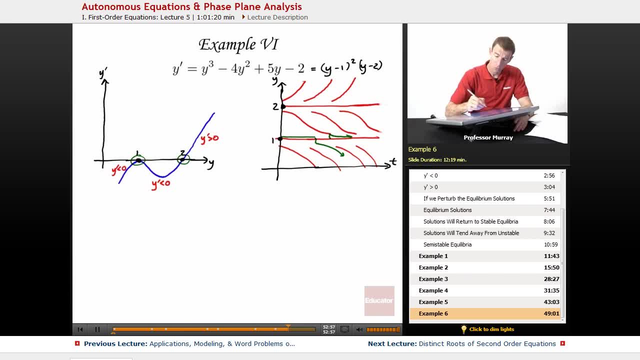 the y equals one again. So what I have there is that y equals one is semi-stable. It depends on which direction you bump it. It's a semi-stable equilibrium. Y equals one is a semi-stable equilibrium because if you bump it a little bit down, 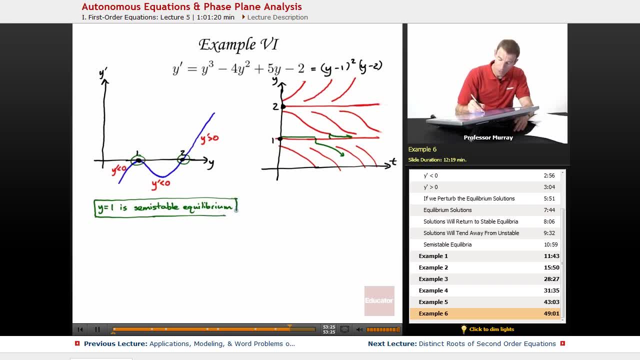 then the solutions run far away. But if you bump it far up, a little bit up, then the solutions run far away. But if you bump it up, then the solutions come back down to y equals one, Y equals two. if I'm on that solution, that equilibrium solution, and I get bumped a little, 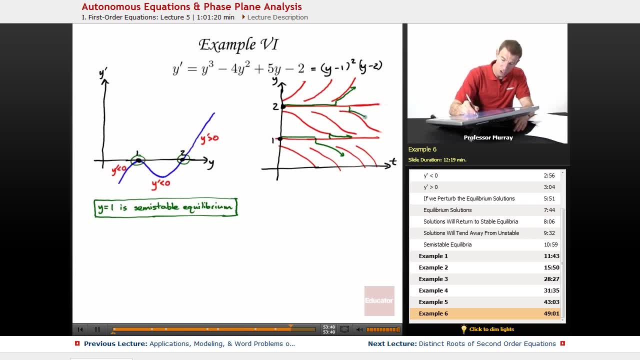 bit. it's going to go far away, And that's true in either direction. It's going to go far away. So y equals two is an unstable equilibrium, because even the slightest bump will send you to a solution curve. that goes far away. 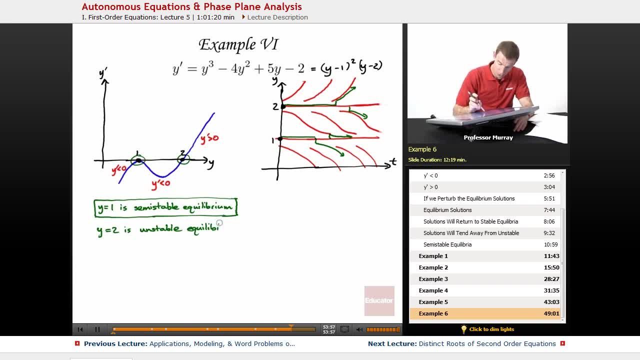 It's going to go far away. It's going to go far away from the equilibrium solution. So, even though it's an equilibrium solution, it's unstable. You would not expect to see it happen in real life, because any slight perturbation will take the solutions far away from that. 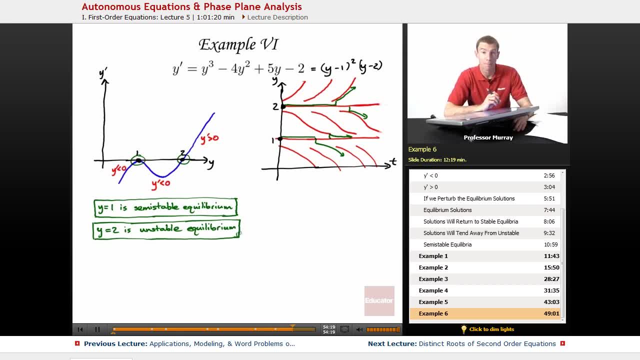 So what we've done is identified our two equilibrium solutions. One was semi-stable and one was unstable. We didn't have any stable equilibrium, We just had a stable equilibrium there. And finally, the question prompt asked us to identify which ranges of initial values 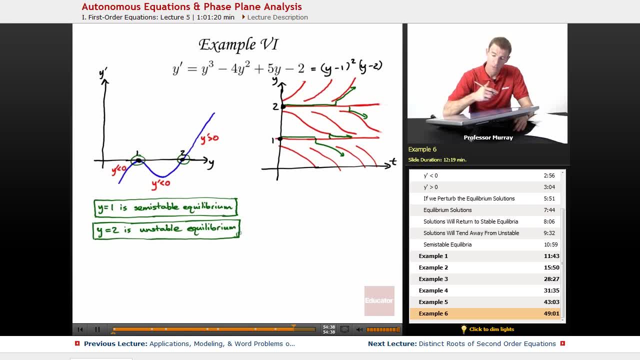 would lead to which limiting behavior for the solution. So let's go back and look at our solution curves. We see that if we're in this region- that's if y is less than if y zero- if we start at a point where y zero is less than zero, 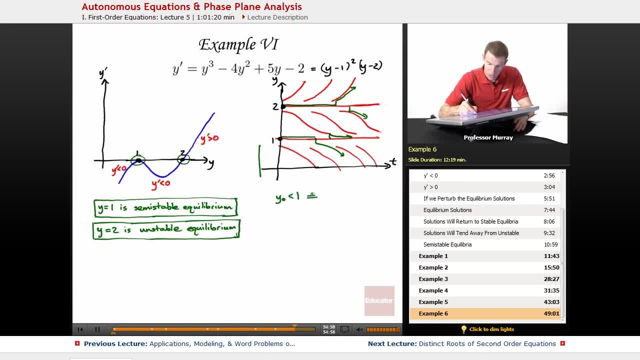 If we start at a point where y is less than 1,, then these solution curves go down to negative infinity. So y goes to as t goes to infinity. as t grows, the y is trending downwards to negative infinity. If we start at 1,, then we're just going to stay at 1.. 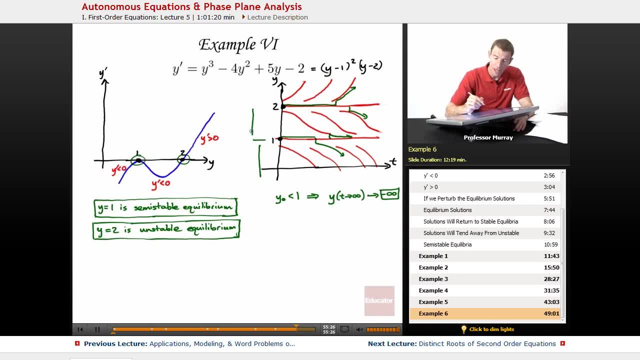 And if we start anywhere in between 1 and 1, we're just going to stay at 1.. in between 1 and 2, then we're going to drift down to 1.. So I'll say, if our initial value of y is 1 or anything between 1 and 2, then y of large values will tend down towards the 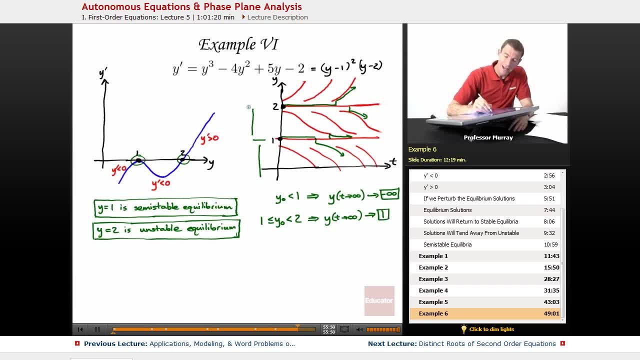 solution at 1.. If we start at 2,, if y not, the initial value of y is 2, then we'll stay exactly on that solution. It would be unstable. so in the real world you wouldn't expect to see this happen. but we would see for large values of time. we would still see y right. 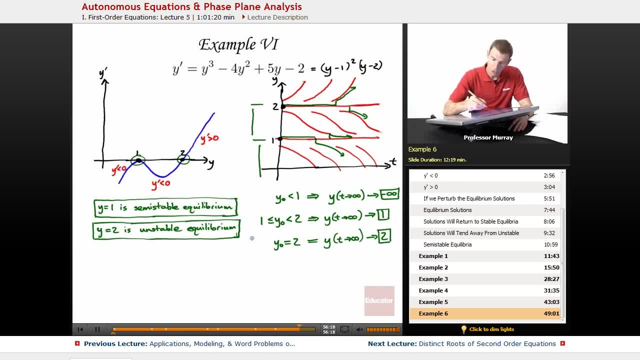 there on that equilibrium solution. And if we start anywhere up here, if y not is anything bigger than 2, then we see that the solution curves go up to infinity. So as we plug in larger and larger values for t, we see that y would increase up to infinity. So now we've identified all the possible things. 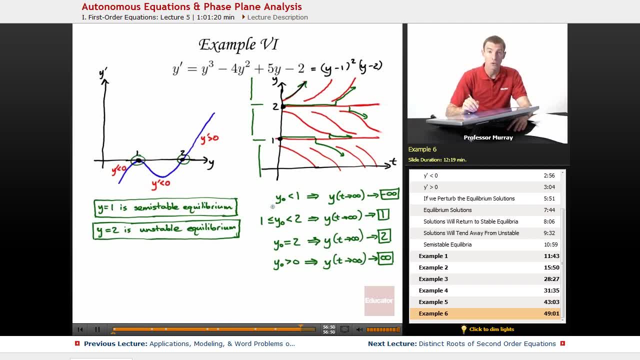 that we need to do to solve this problem. So let me just recap what we did there. We started with the differential equation. We had to do a lot of algebra back in the previous example to factor it down into y-1 squared times y-2.. Once we had that, we drew this: 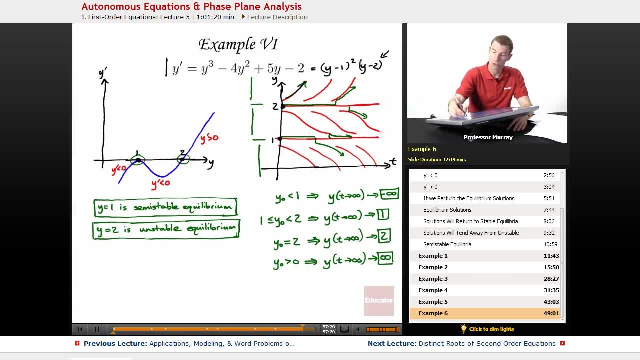 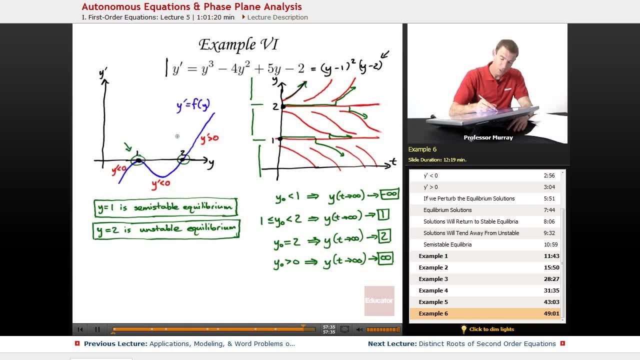 from there we were able to identify the equilibrium solutions at y equals one and y equals two, And then those translated into our equilibrium solutions over here: y equals one, y equals two. That's how we got these two horizontal here. Looking at it in a little more detail, we see that y is negative. sorry, y prime is negative. 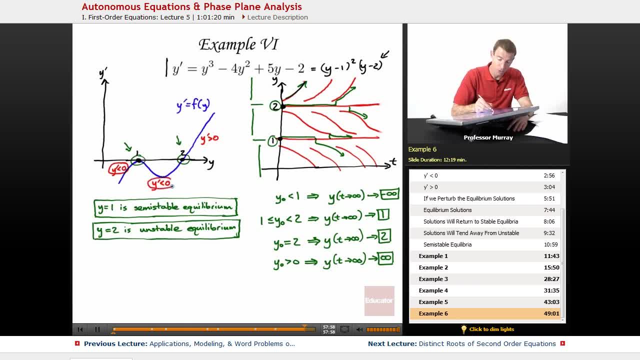 when y is less than 1, y prime is negative when y is between 1 and 2, and y prime is positive when y is bigger than 2.. So that helped us draw these solution: curves sloping downhill when y is less. 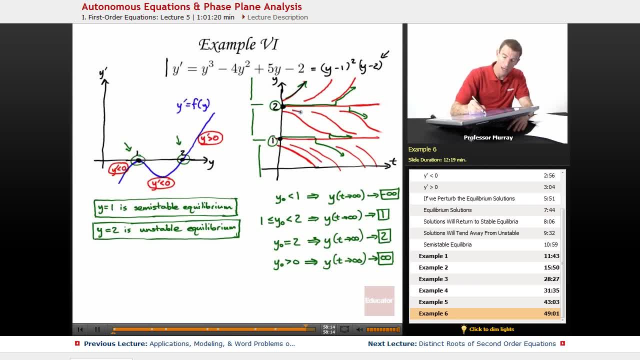 than 1, still sloping downhill when y is between 1 and 2, and then sloping uphill when y is bigger than 2.. So we were able to draw these solution curves and then we can look at those and identify which of our equilibria are stable or unstable. Turned out that y equals 1 was semi-stable. 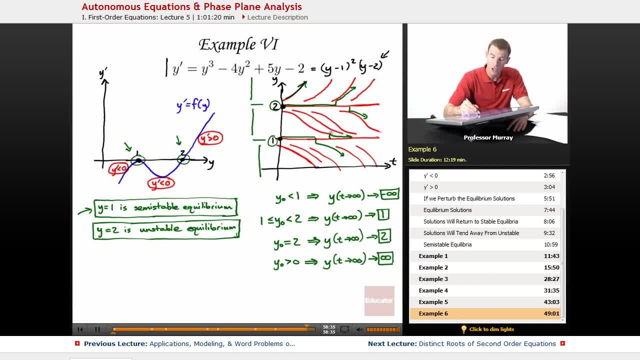 because solution curves sort of approach it on one side. On one side they want to tend towards that solution. On the other side they want to go down. So the answer to this equation is that other side they run away from that solution. So it's stable on one side, unstable on the. 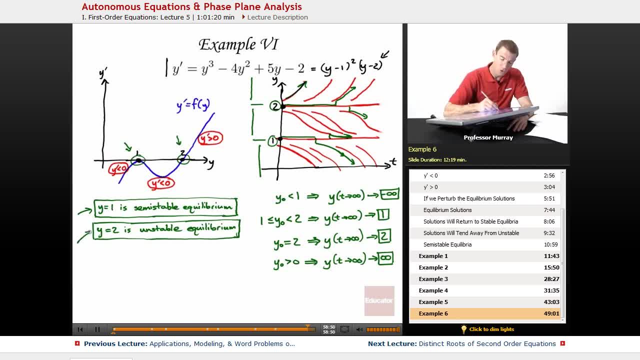 other side, We call it semi-stable. y equals 2 was an unstable equilibrium because the solution curves are drifting away from it. Of course, we could have also noticed that by looking at the original phase plane graph, since at y equals 2, the curve is going upwards. 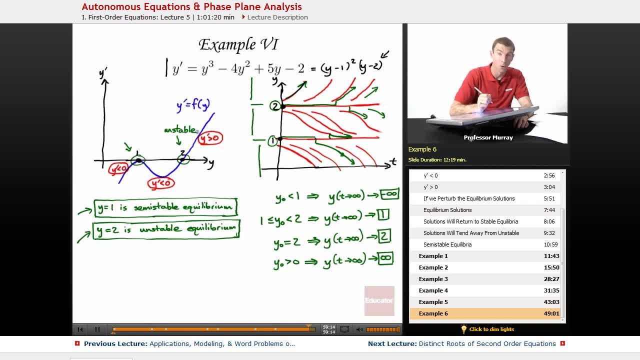 across the horizontal axis. we know that's an unstable equilibrium. And at, y equals 1, since it's just barely touching its tangent to the horizontal axis, we know that's a semi-stable equilibrium. And finally, we were able to look at these solution curves and identify. 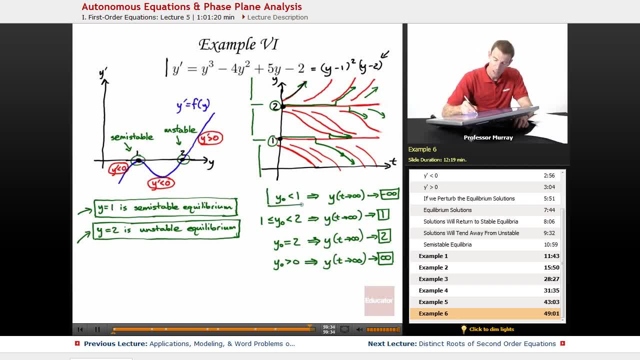 for any possible value of y naught, whether it be less than 1, between 1 and 2, equal to 2, or- Oh, there's a little, Oh, there's a little. There's a small mistake here. I should have said y naught greater than 2.. That corresponds. 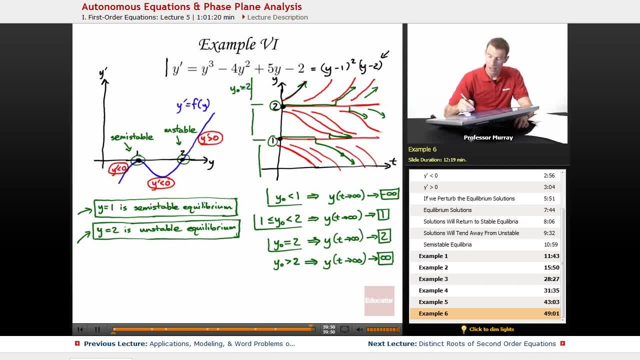 to these values here where y naught is greater than 2.. So we were able to look at those and identify for any possible range where the solution curves will end up. If you're less than 1, you're going to be going down to negative infinity. If you're between 1 and 2, you're 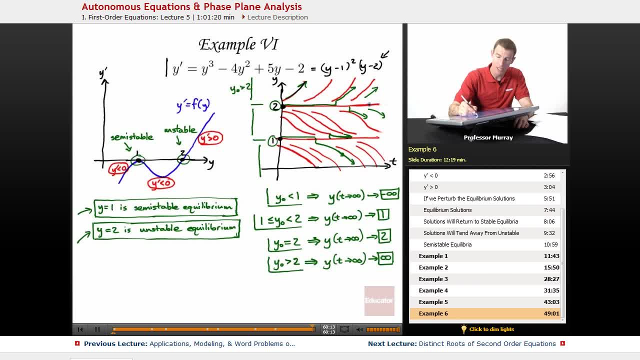 going down to negative infinity. If you're at 2, then you're just going to keep going exactly at y equals 2.. But if you're anything bigger than 2, then you're going to be going up to positive infinity. So the whole point of this study of autonomous equations and 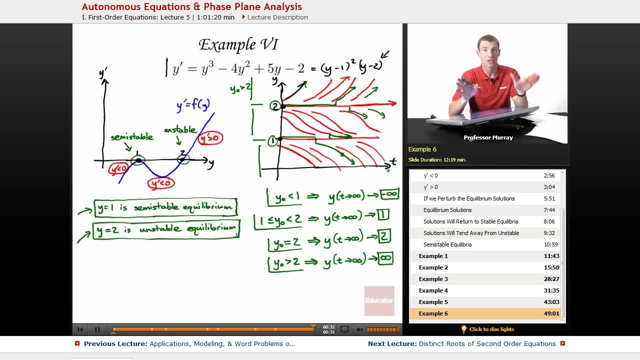 phase plane analysis is that nowhere in any of this did we actually solve the differential equations. Instead, we had this autonomous equation where we had no x's or y's and there were t's on the right-hand side, just y's, And so from that we were able to produce. 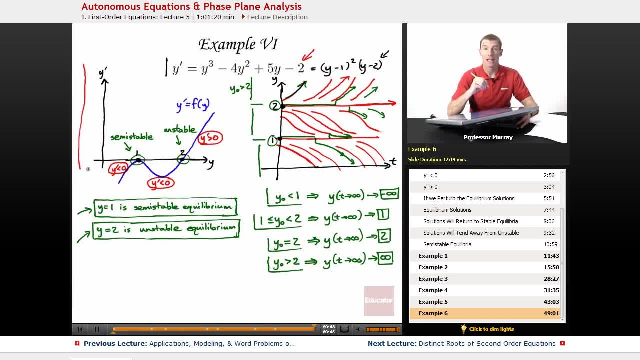 a graph of y prime versus y And from there we were able to really get a lot of information about the actual solutions y versus t. We were able to figure out the equilibrium solutions, whether they're stable or unstable, where the other solutions go and where you would.